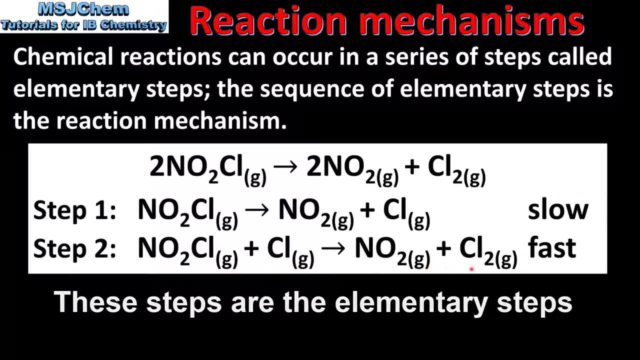 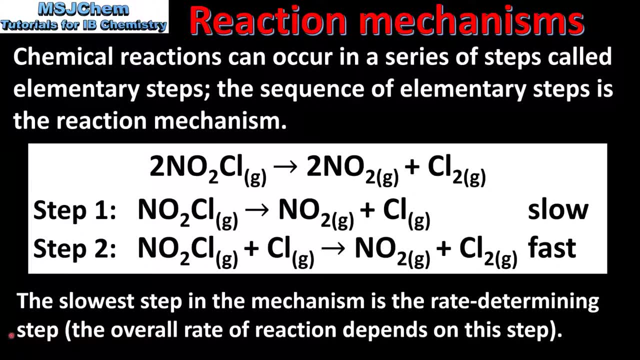 to form nitrogen dioxide and a molecule of chlorine. We can also see that step one is labeled as slow and step 2 as fast. The slowest step in the reactionARE mechanism is the rate determining step. the overall rate of reaction depends on this step. so in this reaction mechanism, step one is the rate determining step. 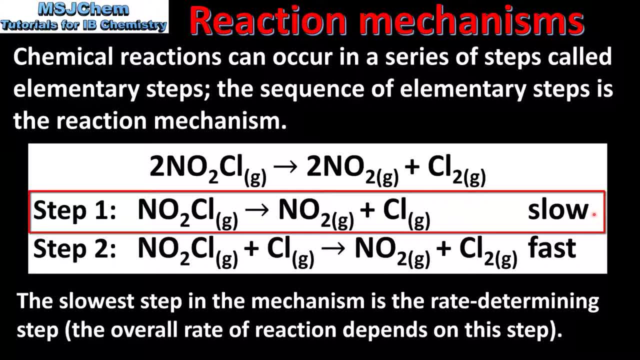 the overall rate of the reaction depends on this step only. it's important to note that the reaction mechanism is only a theory of how the reaction takes place. therefore, we can never prove that the reaction mechanism represents the actual chemical change taking place. so next we look at the three criteria that need to. 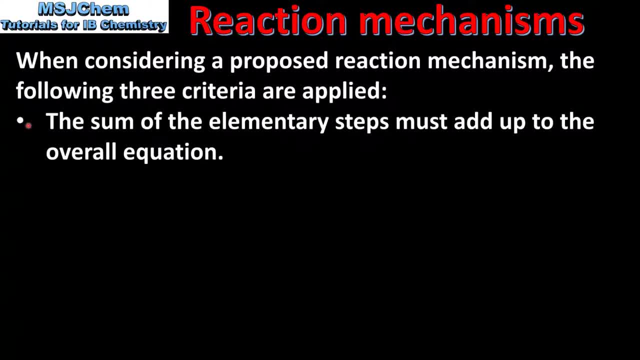 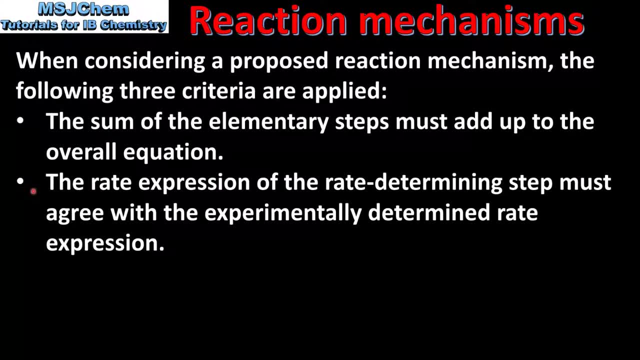 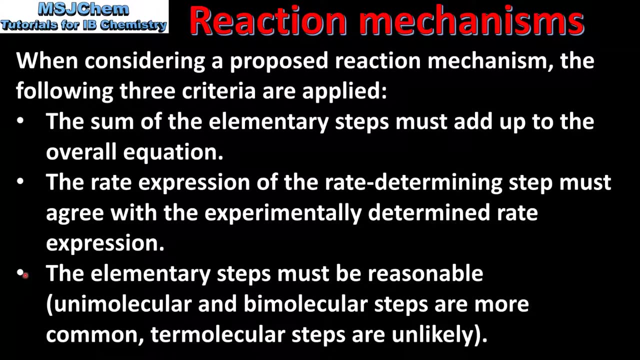 be applied when considering a reaction mechanism. the first is that the sum of the elementary steps must add up to the overall equation. the second is the rate expression of the rate determining step must agree with the experimentally determined rate expression. and the third is that the elementary steps must be: 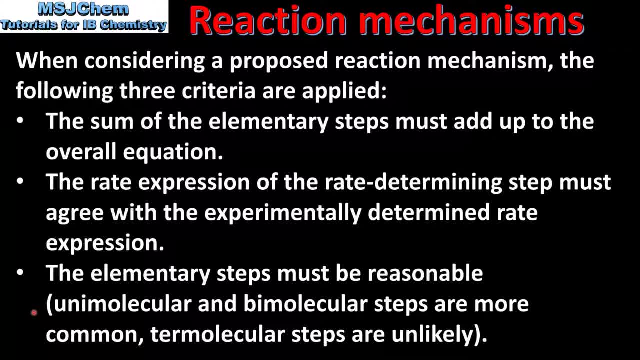 reasonable. unimolecular and bimolecular steps are more common, whereas termolecular steps are more common and unimolecular steps are more common and unimolecular steps are unlikely. so next we'll apply these three criteria to the reaction mechanism in the previous slide. so the first step is to determine. 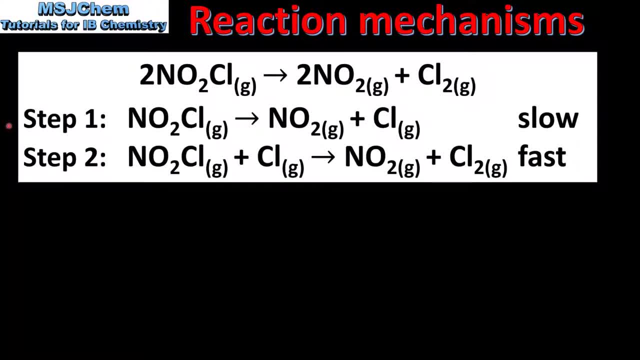 if the elementary steps add up to the overall equation. to do this, we need to identify any reaction intermediates in the reaction mechanism. if we look at the reaction mechanism, we can see that the chlorine atom is a reaction intermediate. it is produced in one step and consumed in the next step. 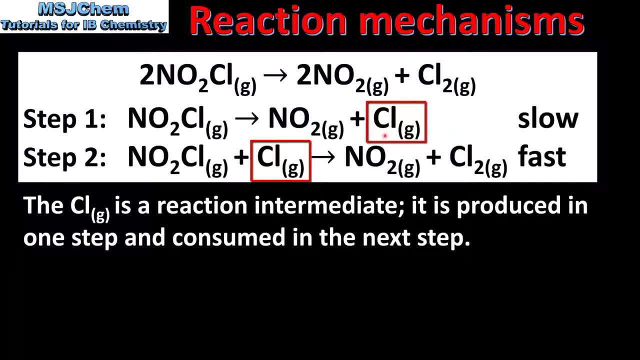 so here we can see that the chlorine atom is produced in step one and it's consumed in step two. reaction intermediates do not appear in the overall equation, therefore they cancel out. we are now left with 2NO2Cl in the reactants and 2NO2 and 1Cl2 in the products. so from this we can see that 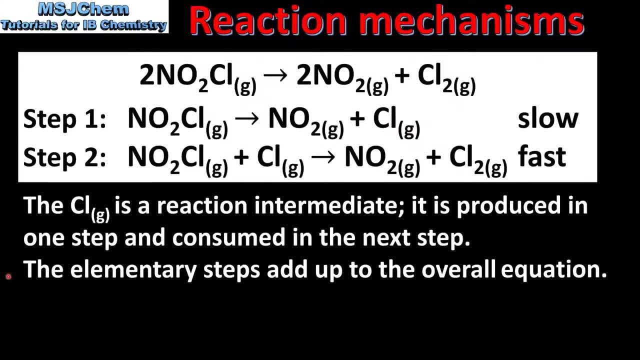 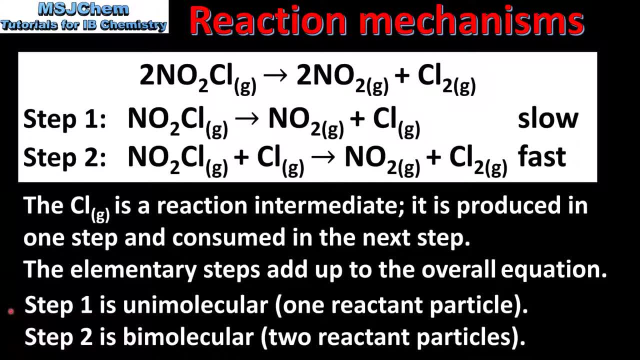 the elementary steps add up to the overall equation. so next we look at the molecularity of each elementary step. step 1 is unimolecular with one reactant particle, and step 2 is bimolecular with two reactant particles. therefore, both elementary steps are 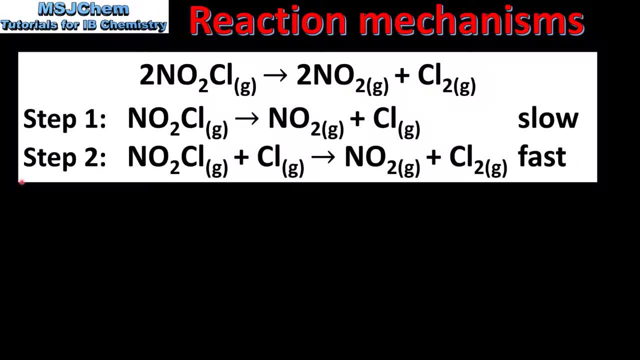 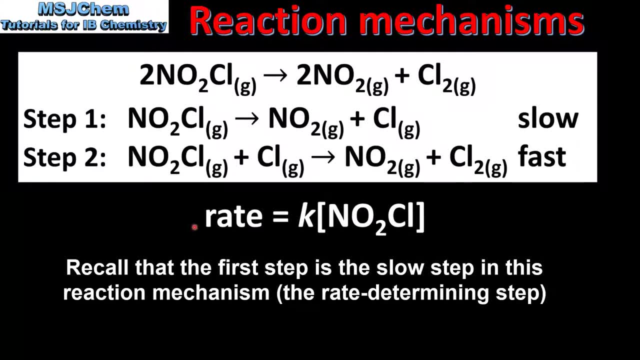 probable. finally, we'll see if the rate expression determined from the rate determining step agrees with experimental data. so here we have the rate expression that was determined from the first step, which is the rate determining step. according to this rate expression, the reaction is first order with respect to nitrile. 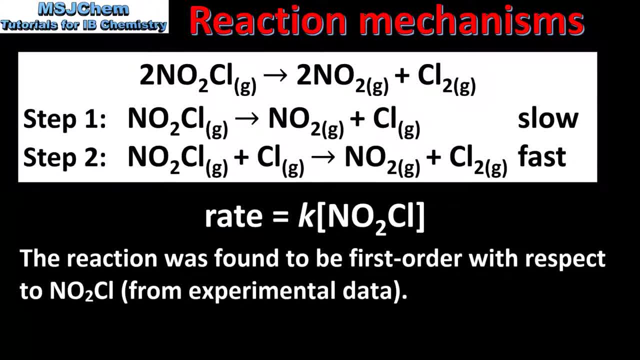 chloride and the reaction was found to be first order with respect to nitrile chloride from experimental data. so from this we can see that the rate expression determined from the rate determining step agrees with the experimentally determined rate expression. so to summarize, this reaction mechanism has 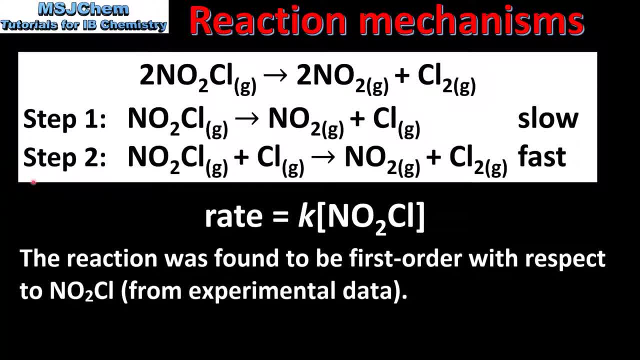 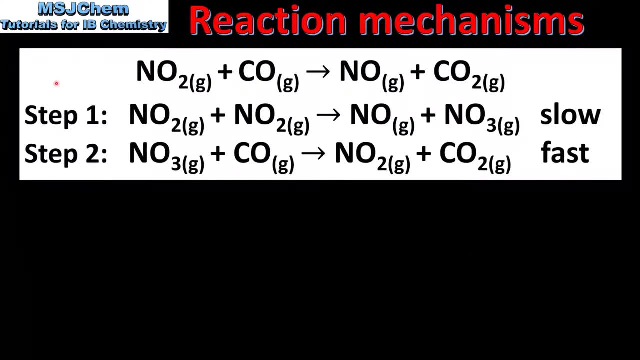 satisfied all three criteria. however, although we have evidence that supports this reaction mechanism, we can never be sure that it represents the actual chemical change taking place. in our next example we look at the proposed reaction mechanism for this reaction. just like in the previous example, we have a two-step reaction. 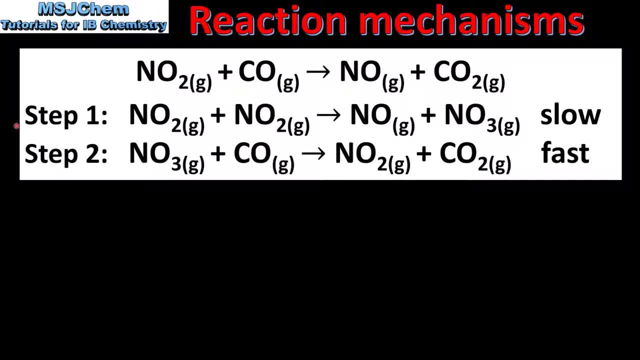 mechanism, with a slow step being the first step, which is the rate determining step. so we'll start by seeing if the elementary steps add up to the overall equation. so in step one the no3 is produced and it's consumed. in step two, therefore, the NO3 is a reaction intermediate and is crossed out. 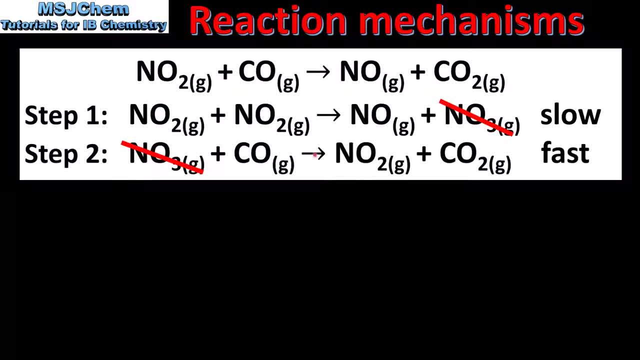 We also have one NO2 in the products in step 2 and two NO2s in the reactants in step 1.. So we can cross out one NO2 from the reactants in step 1 and the NO2 from the products in. 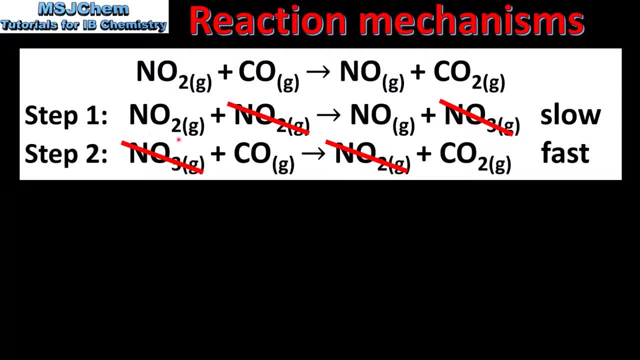 step 2.. So we are left with one NO2 and one CO in the reactants and one NO and one CO2 in the products. Therefore, the elementary steps add up to the overall equation. Next we look at the molecularity of each step. 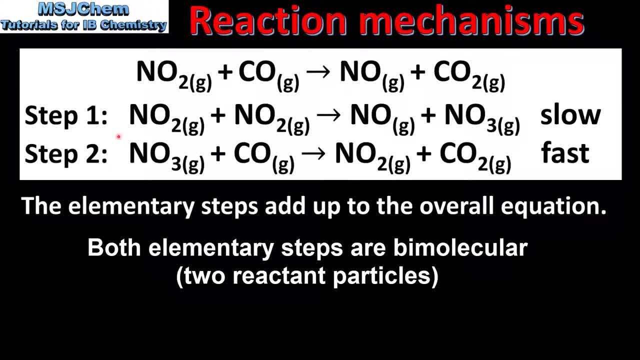 So in both elementary steps we have two reactant particles. therefore they are both bimolecular. Finally, we'll see if the rate expression that's determined from the rate determining step agrees with the experimentally determined rate expression. So this is the rate expression determined from the rate determining step, which is the 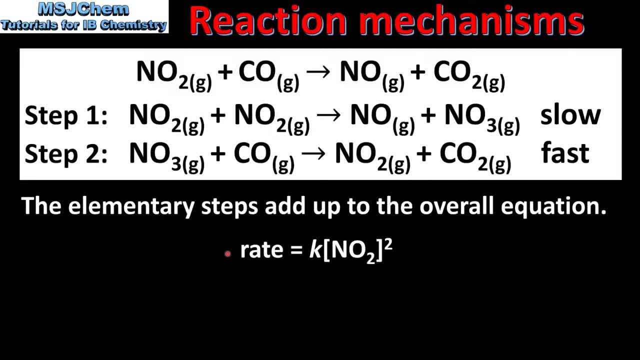 first step. According to this rate expression, we have two reactant particles. So we can see that the reaction is second order with respect to NO2 and the reaction was found to be second order with respect to NO2 from experimental data. So we can see that the rate expression determined from the slow step agrees with the experimentally. 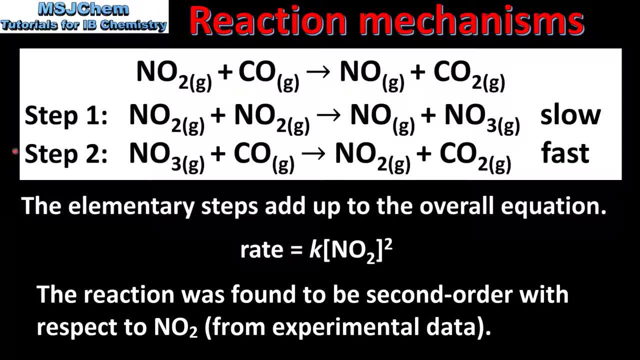 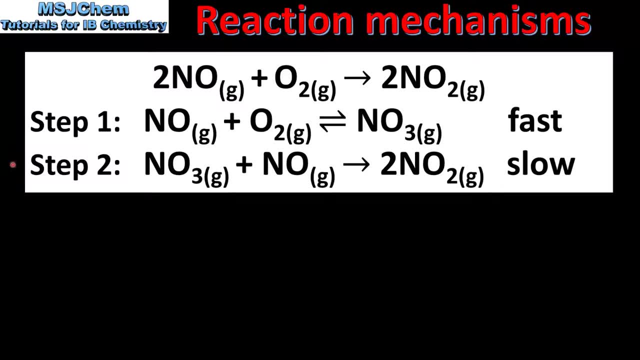 determined rate expression. So once again, we can see that this reaction mechanism satisfies the three criteria. Therefore, this is a possible reaction mechanism for the reaction. In our next example We have a reaction. The reaction mechanism with the second step is the slow step. 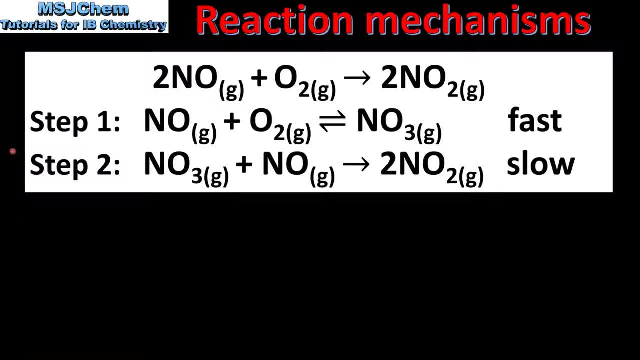 So we'll start by identifying any reaction intermediates. We can see that the NO3 is produced in step 1 and it's consumed in step 2. Therefore it cancels out. So we are left with 2NO plus O2 in the reactants and 2NO2 in the products. 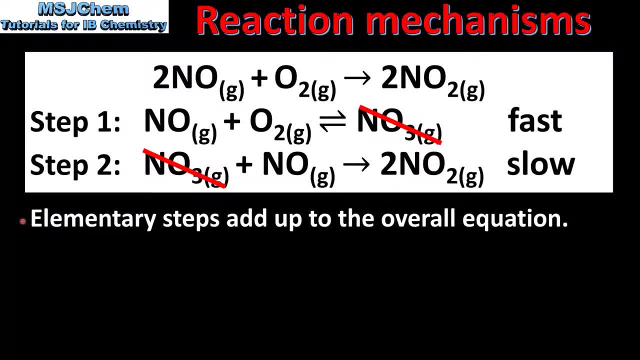 So from this we can see that the elementary steps add up to the overall equation. If we look at the molecularity of the reactants, we can see that the NO3 is produced in step 1.. If we look at the molecularity of the elementary steps, we can see that both steps are bimolecular. 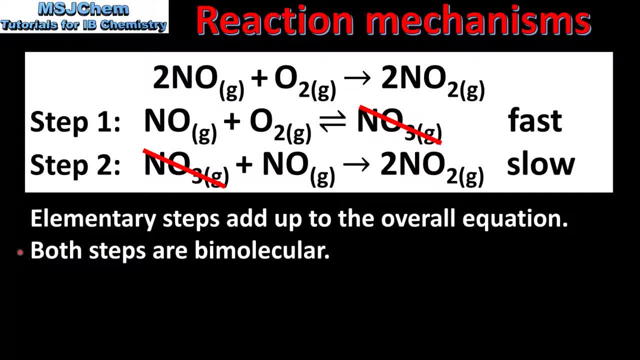 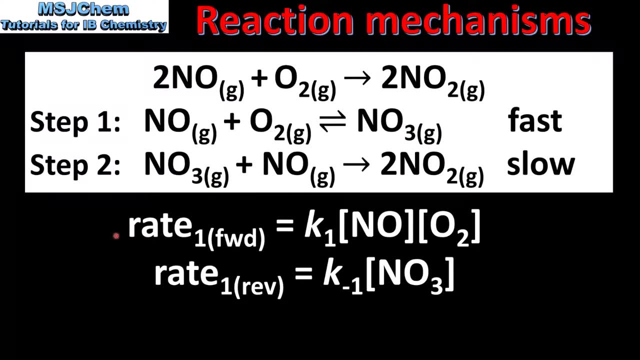 The final criteria is to see if the rate expression determined from the slow step matches the experimentally determined rate expression. Because the second step is the slow step, we need to take a slightly different approach to this example. We start by writing the rate expressions for the forward reaction in step 1 and the reverse 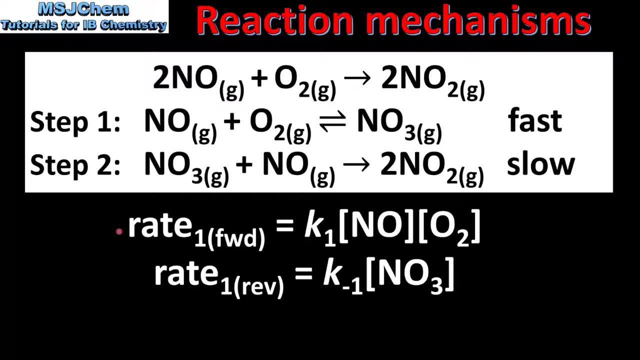 reaction in step 1.. So here we have the rate expression for the forward reaction. So we can see that the reaction in step 1 matches the reaction in step 2.. And here we have the rate expression for the reverse reaction. Next we write the rate expression for step 2.. 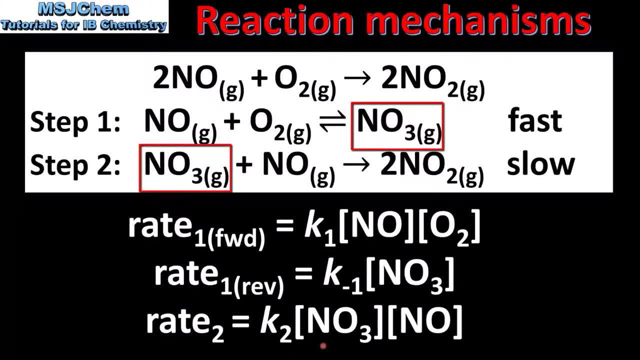 If we look at the rate expression for step 2, we can see that it contains the NO3, which is a reaction intermediate. Overall rate expressions cannot include reaction intermediates, so we need to eliminate the NO3 from this rate expression, To eliminate the reaction intermediate from the rate expression. we need to express the. 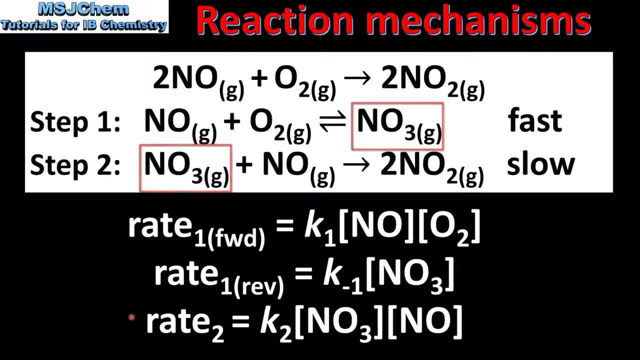 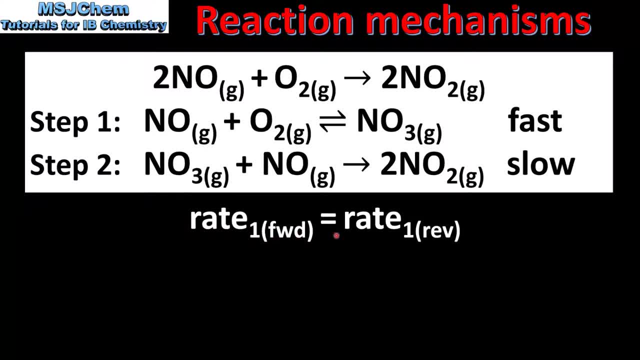 concentration of NO3 in terms of reactants: reactants. So by looking at step 1 we can see that it reaches equilibrium, with a rate of the forward reaction is equal to the rate of the reverse reaction. So here we have the rates of the forward and reverse reactions written in terms of. 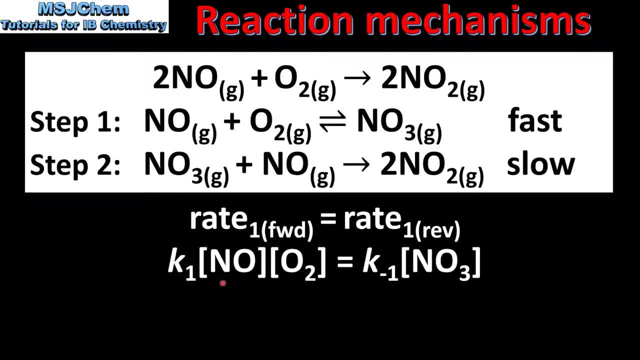 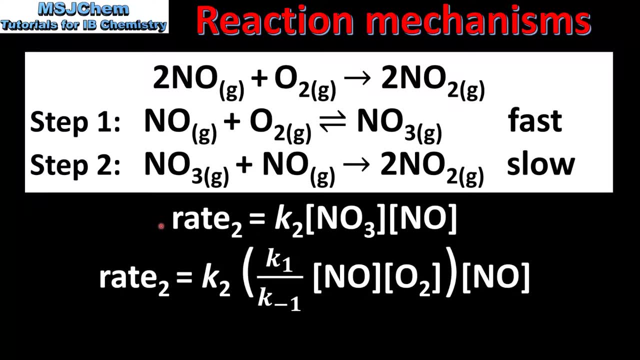 the rate constant and the concentrations of reactants. Next, we express the concentration of NO3 in terms of reactants, which we can see here. The next step is to substitute in for the concentration of NO3 in the rate expression for the second step And finally, this gives us the rate. 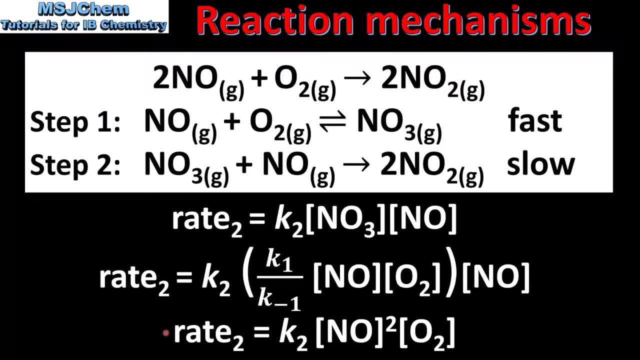 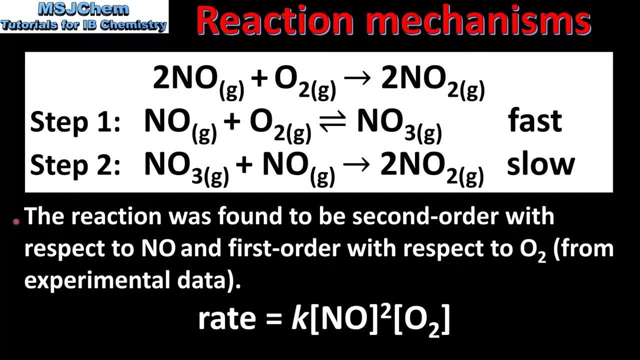 expression for the second step. So, according to the rate expression determined from the rate determining step, which in this example is the second step, the reaction is second order with respect to nitrogen monoxide and first order with respect to oxygen. From experimental data, the reaction was found: 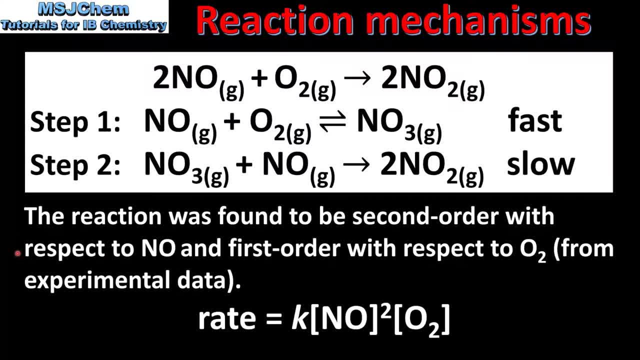 to be second order with respect to nitrogen monoxide and first order with respect to oxygen. So here we can see the experimentally determined rate expression. So the rate expression that was determined from the slow step agrees with the experimentally determined rate expression. So to 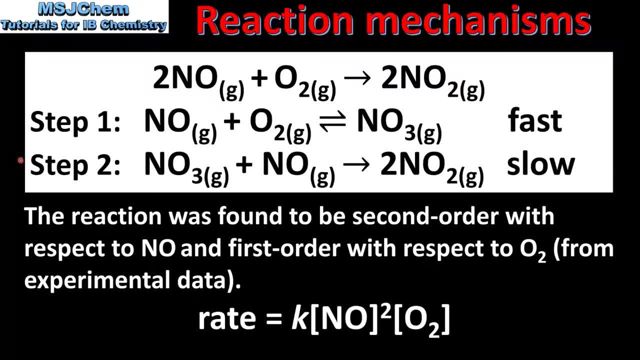 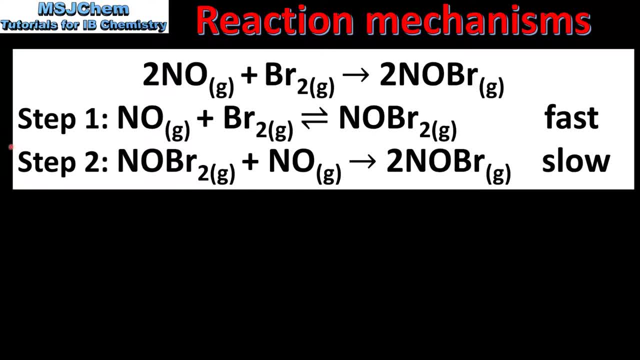 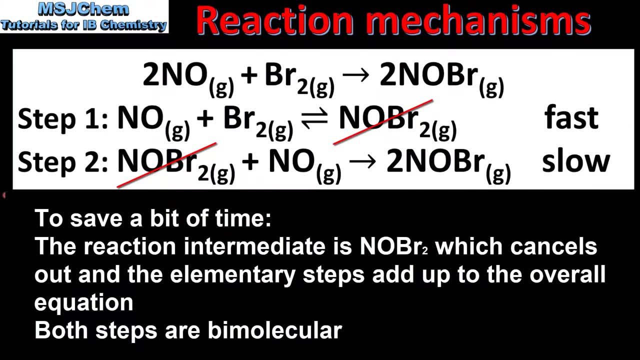 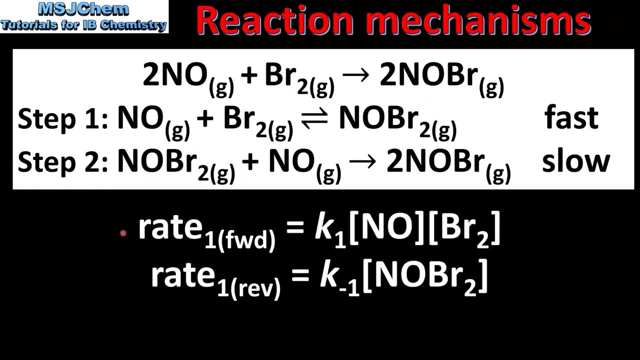 summarize: this reaction mechanism satisfies all three criteria. Next, we look at one more example where the first step is the fast step and the second step is the slow step. So, like in the previous example, we start by writing the rate expressions for step one, for the forward and reverse reactions. We then write the rate. 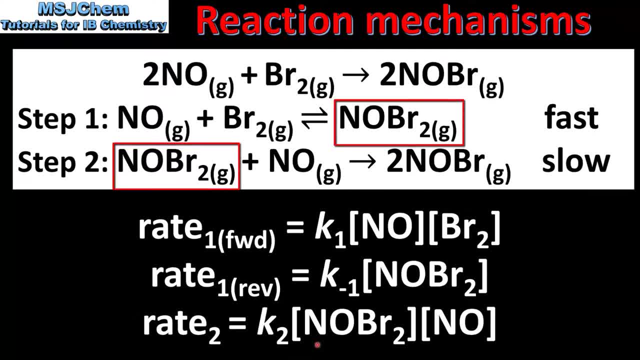 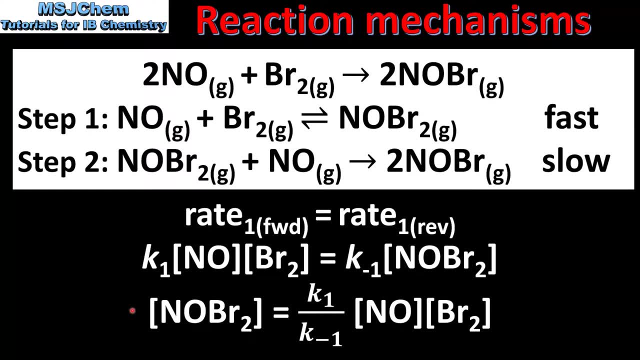 expression for the second step. As we can see, the rate expression for the second step involves a reaction intermediate. The overall rate expression cannot include reaction intermediates. therefore, we need to eliminate it from the rate expression, To eliminate the NOBr2, which is the 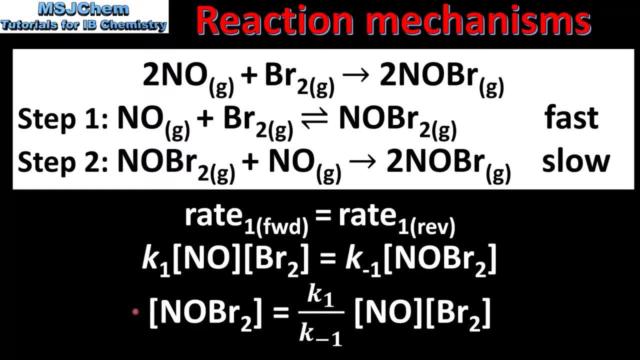 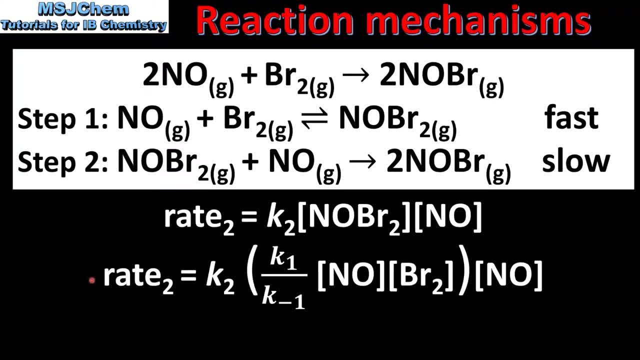 reaction intermediate. we need to express it in terms of reactants, Which is this step. here. We then substitute for the concentration of the NOBr2 in the rate expression for the second step And finally we arrive at the rate expression for the second step, which you can see here. 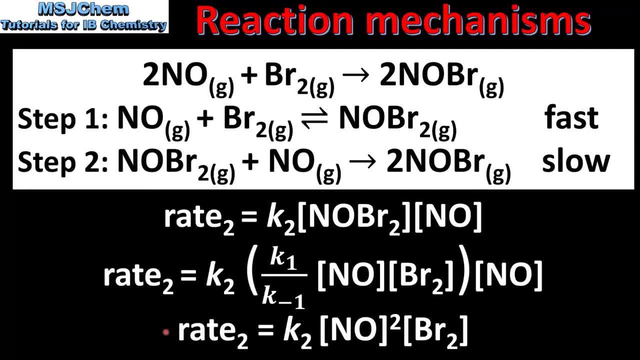 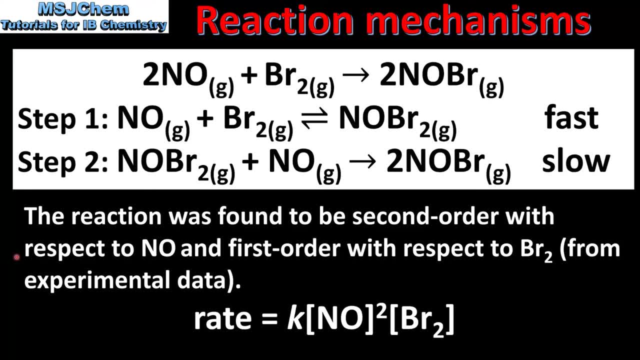 So next we'll compare this rate expression to the experimentally determined rate expression. So the reaction was found to be second order with respect to nitrogen monoxide and first order with back to bromine. So to summarize, the rate expression determined from the slow step. 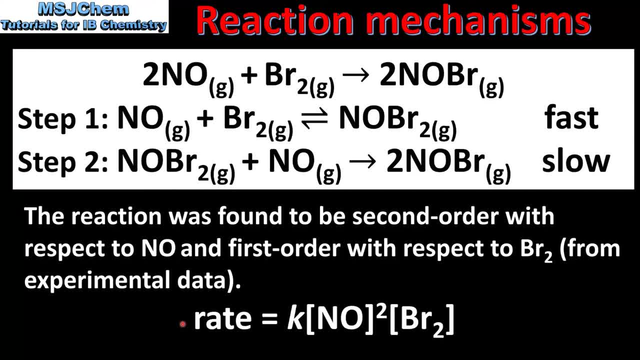 which is the rate determining step, agrees with the experimentally determined rate expression and this reaction mechanism satisfies the three criteria.